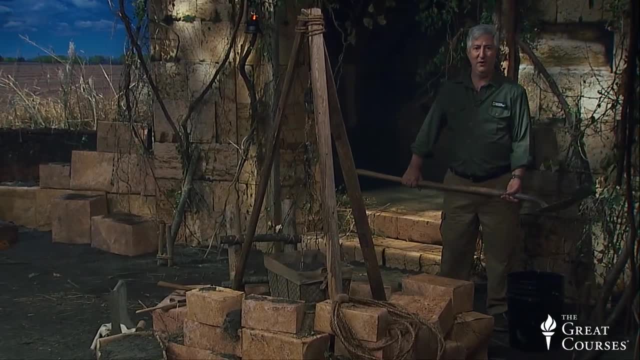 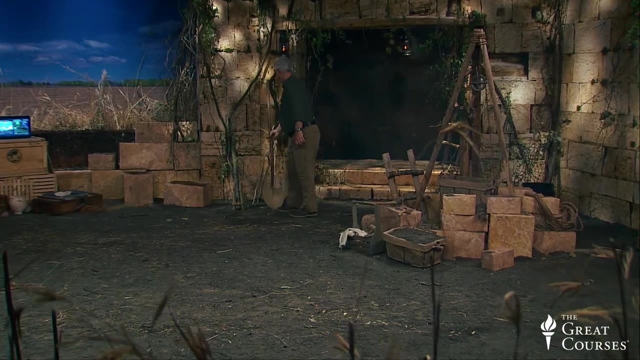 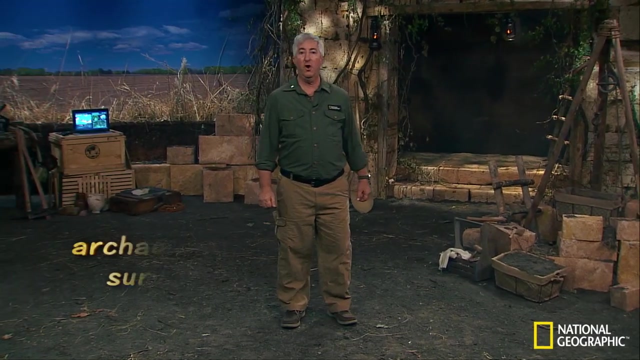 I'm frequently asked: how on earth do you know where to dig? Well, that is a great question, And it actually bears on some of the tools and the methods that archaeologists employ. So I'm going to talk about the concept of archaeological surveying. that is the 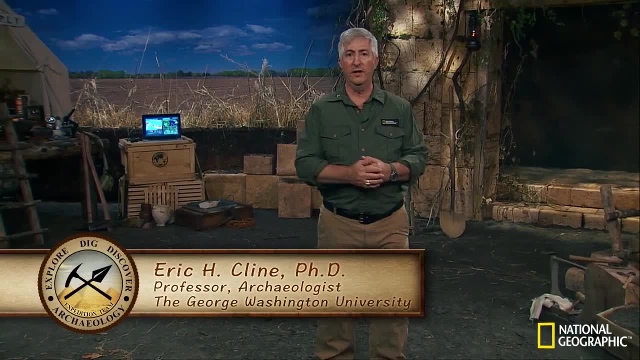 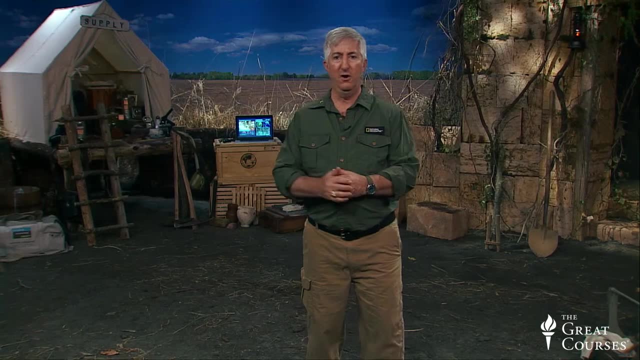 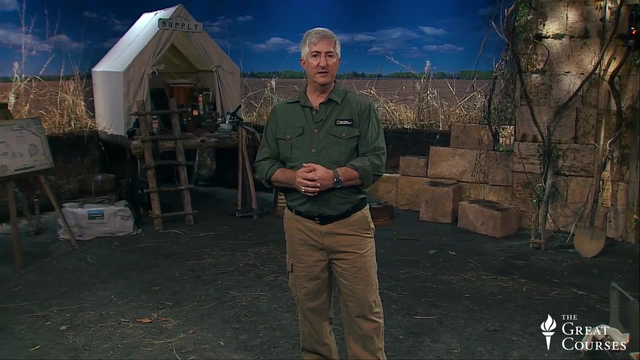 process of looking for sites. I'm also going to introduce you to the various types of remote sensing that are now used by archaeologists. Now, first of all, let's define what we mean by a site, because these come in all shapes and sizes Within their textbook In the Beginning. 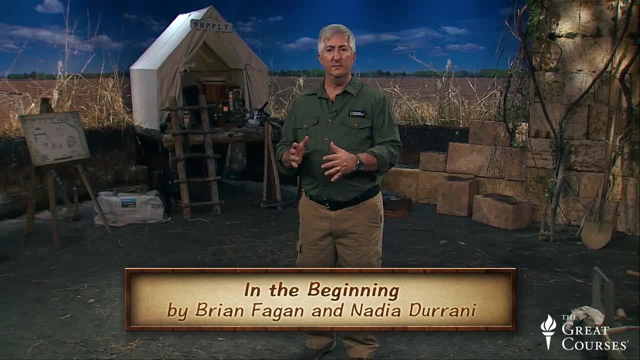 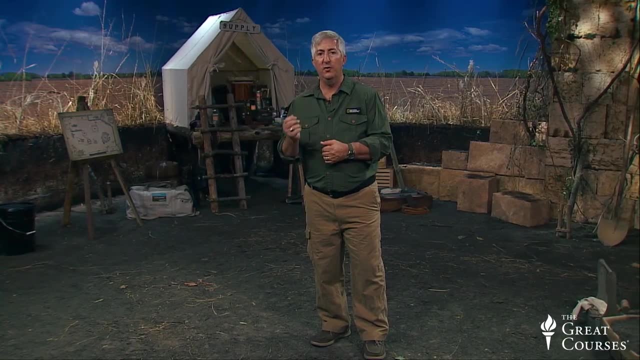 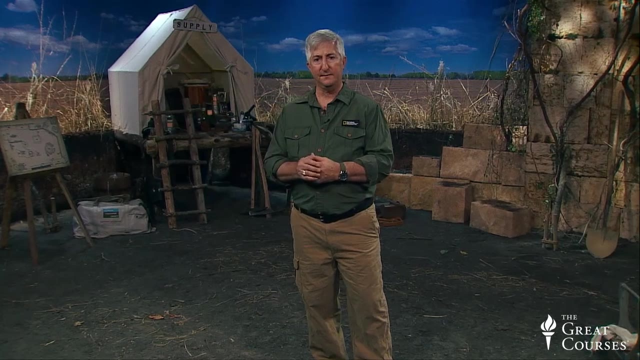 Brian Fagan and Nadia Durrani define a site simply as a place where traces of past human activity can be found, And these are normally identified by the presence of artifacts. Some of them are pretty obvious, For example, when you look at the Athenian Acropolis or a huge mound like Megiddo in 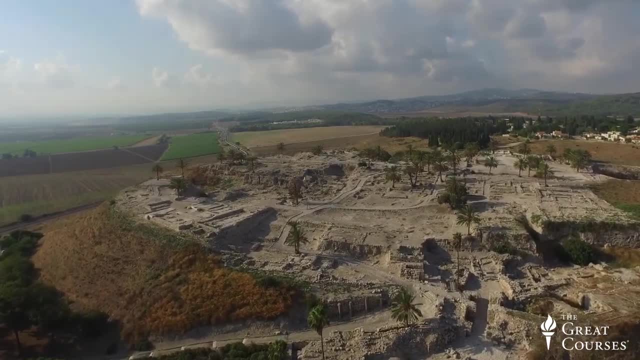 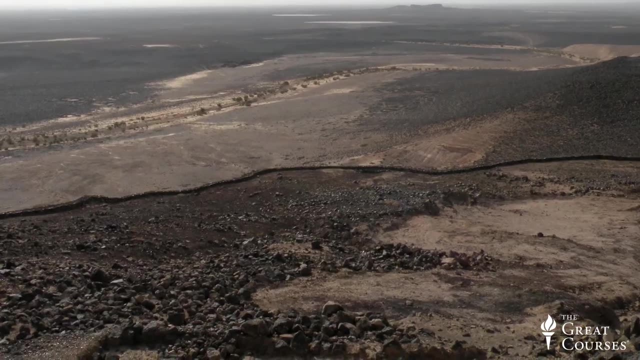 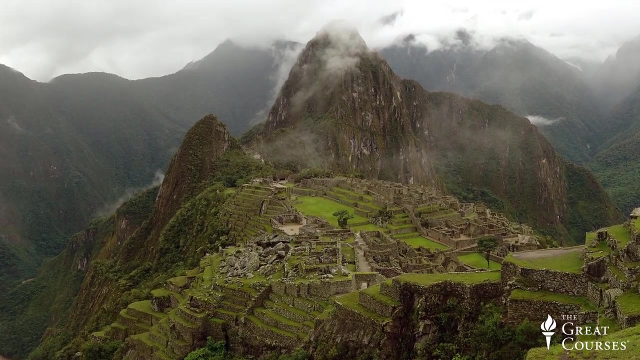 Israel. you know that you're looking at an ancient site, But others can be very tiny and almost indiscernible. A site can be as small as a scatter of flakes where somebody once made a stone tool, or as large as Machu Picchu in Peru. The trick is to find the ones. 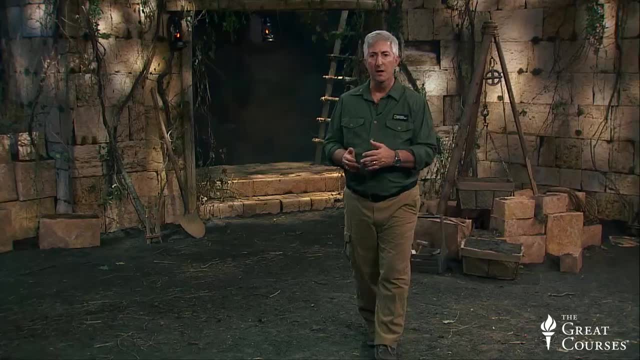 that aren't so easy to detect. There are two basic ways to find sites. Do you want to find sites? You can go to Google and search for sites. You can go to Google and find sites. You can see sites as pretty as a yellow dot. Do you want to search for sites? There are. different ways. You can search for sites like Mount Arbiter and Mount Hagia de Ina. the Mount Arbiter is a place where real estate is being used for construction, land access and even for mining and mining sites, And you can find sites that are helps to find. 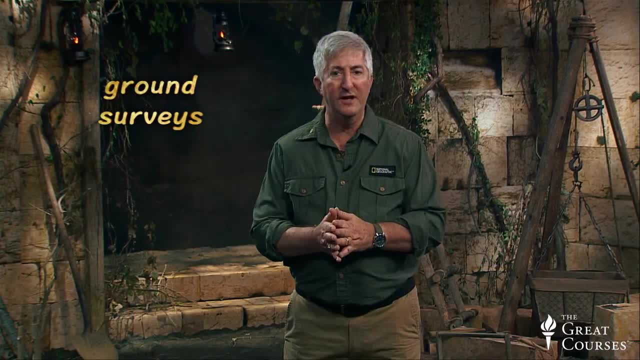 sites. You can also find sites where people were killed or murdered. The word site can some times be a bit more complex, but it isn't always just about a city, but it can also be a lot more complicated. There are several ways you can find sites. For example, you can search for sites such 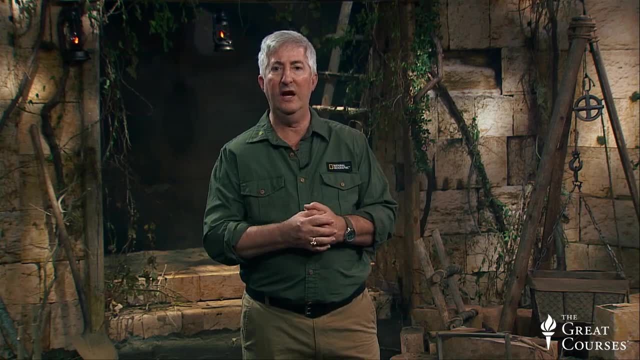 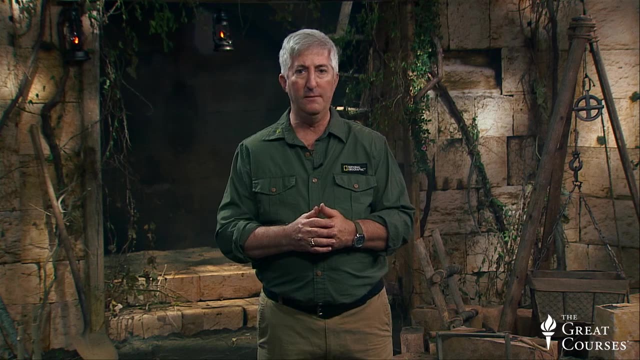 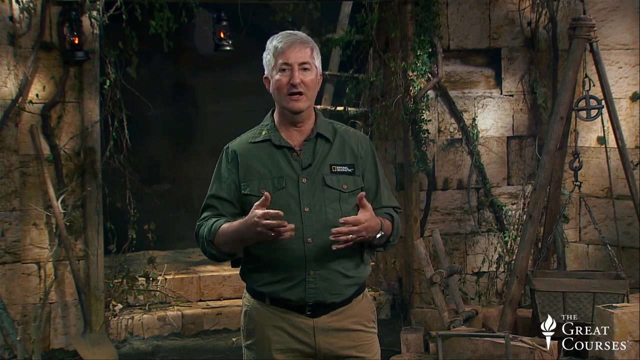 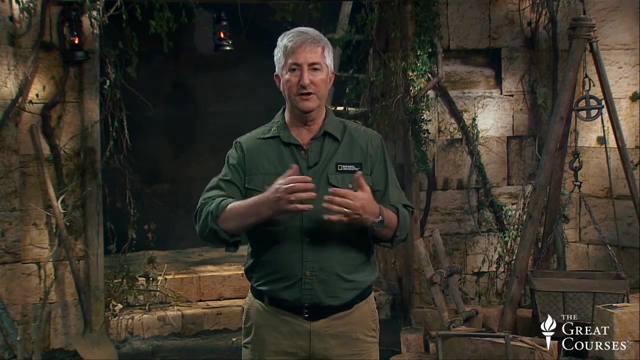 as the Black Sea. You can search for sites that have very little or noThen the different types of questions than you can when you're digging a single site. So, for instance, you might want to investigate how intensively a specific area in Greece was. 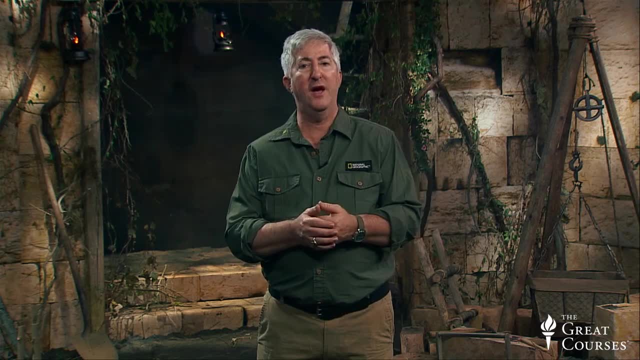 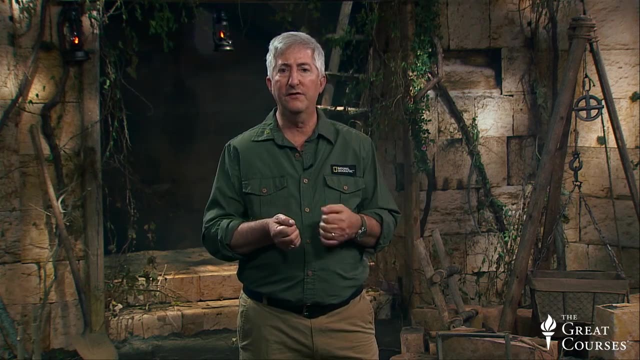 occupied during the Bronze Age. Did that settlement pattern change during the following Dark Ages, And what happened when things began to return to normal and we get into the eras of Archaic and then Classical Greece? What happened in the region when the Romans arrived? What was? 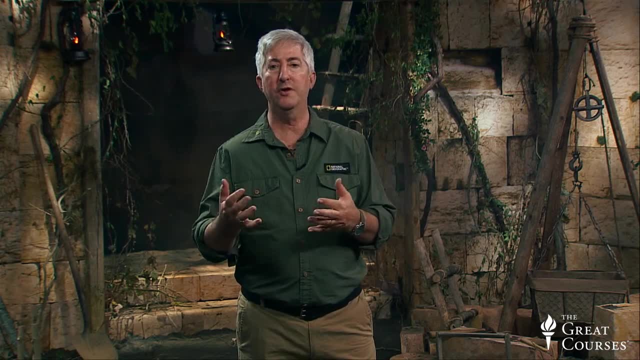 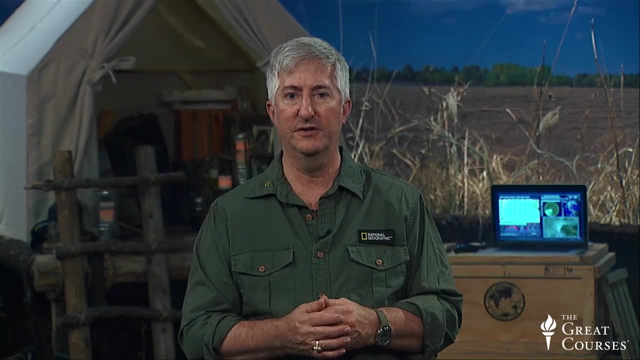 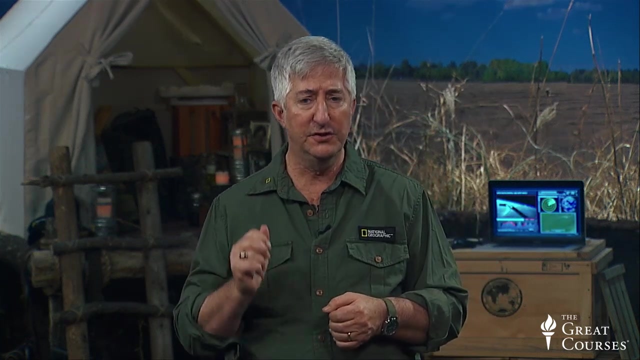 it like in the Byzantine period, And how about the Ottoman period or the modern period? Ground surveys can help you answer these kinds of questions. By doing surveys and identifying the various sites from different periods in the area, you can actually construct a history of. 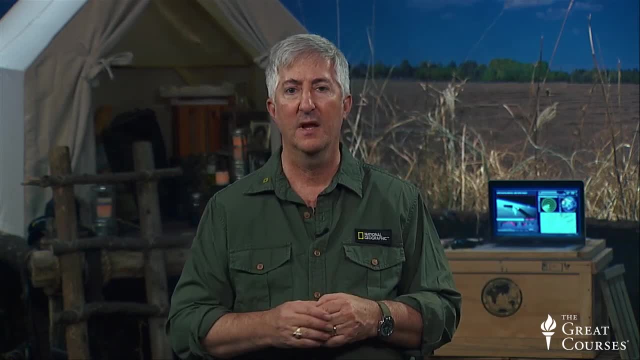 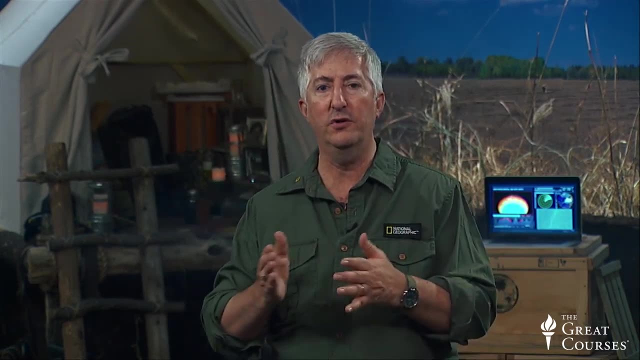 the region without ever digging at a single site. Many surveys, though, do lead into an excavation afterward, as the archaeologists zoom in on one or more of the sites- The most promising new sites that they've just found- and get a permit to dig there. 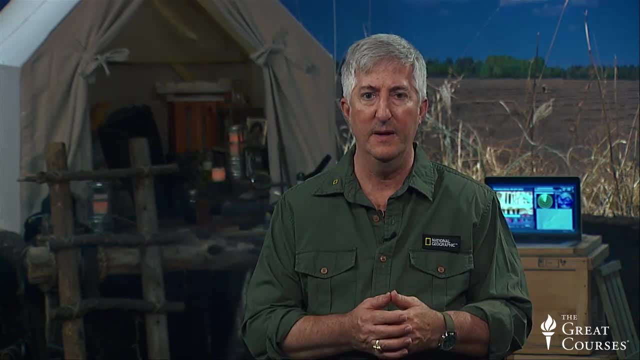 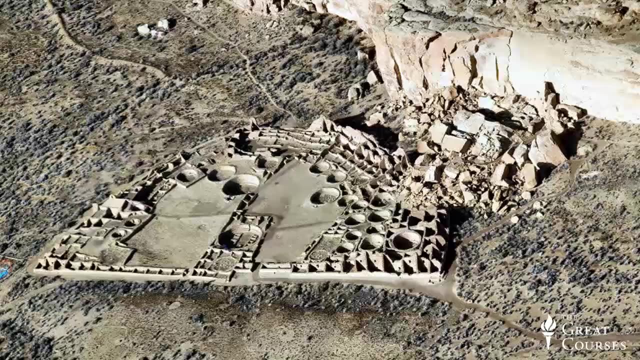 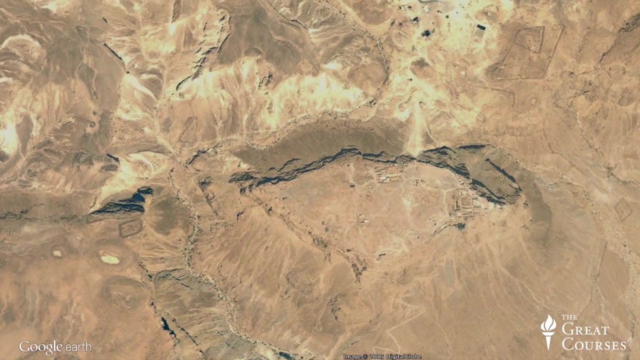